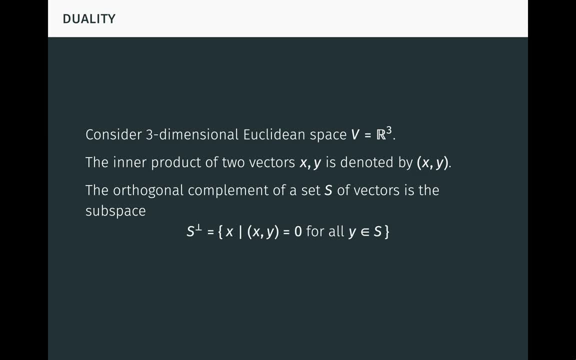 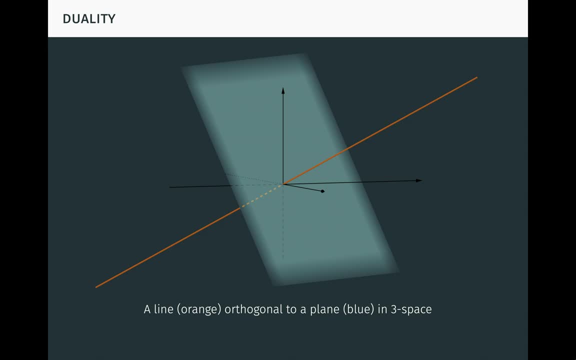 that x times y is equal to zero for all vectors y and s. We can visualize this easily Here. for example, the orange line is the orthogonal complement of the blue plane and vice versa. It's useful to keep this picture in mind. 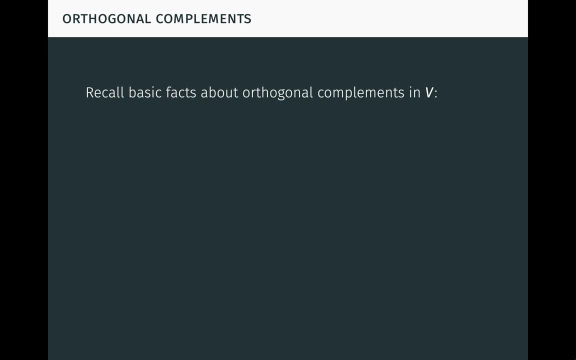 There are a number of basic facts about orthogonal complements in R3, which you've probably seen before. Take a moment to pause the video and think through these Here. the sum u plus w is the smallest subspace containing both u and w. 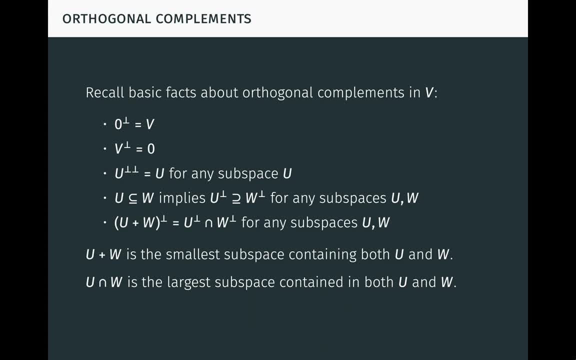 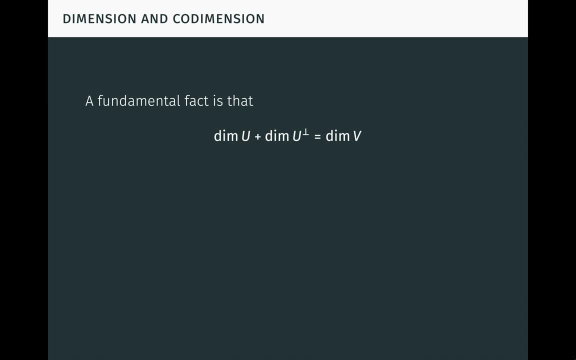 The intersection u intersect w, is the largest subspace contained in both u and w. A fundamental fact is that the dimension of a subspace, u plus the dimension of the subspace u-complement, is equal to the dimension of v, which in this case is 3.. For example, if u is a, 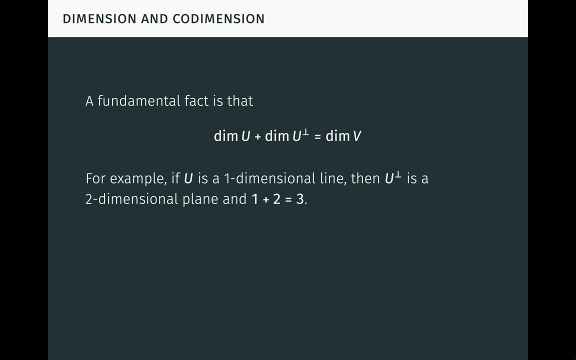 one-dimensional line, then u-complement is a two-dimensional plane, as we saw in the picture, and certainly 1 plus 2 equals 3.. If we define the codimension of a subspace, w, to be the dimension of v minus the dimension of w, this just says that the dimension of u is the codimension of u-complement. 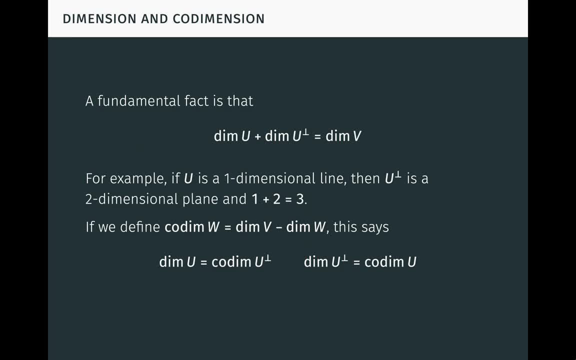 and the dimension of w is the dimension of the subspace w. The dimension of u-complement is the codimension of u. Now consider a familiar dimension, inequality, which says that the dimension of the sum of two subspaces is, at most the sum of their dimensions. For example, if u and w are lines, 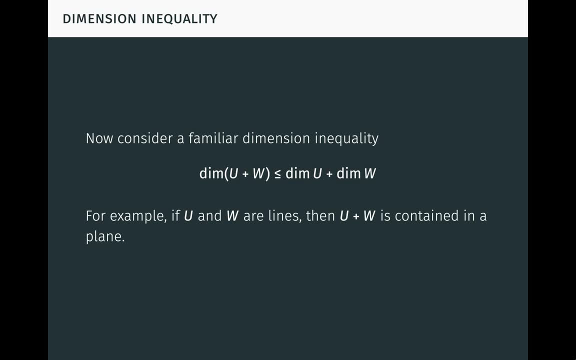 then their sum is contained in a plane. It's possible to compute the dimension of the sum exactly, but we don't need to. for this simple example, We can immediately obtain from this inequality a corresponding codimension, inequality which says that the codimension of an intersection of two subspaces 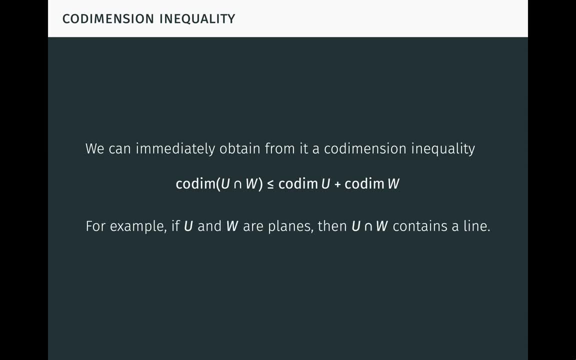 is at most the sum of their codimensions. For example, if u and w are planes, then their intersection contains a line To prove this. first observe from the basic facts earlier that u-intersect w is u-complement-complement-intersect-w-complement-complement. 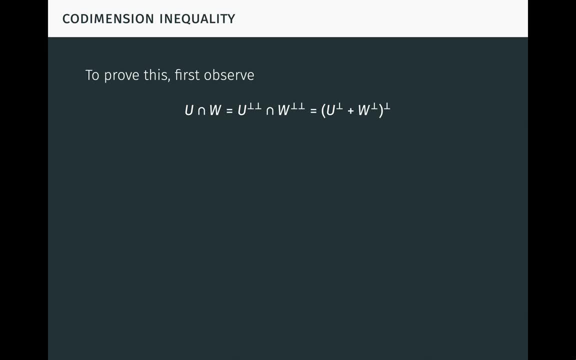 which is just the complement of the sum u-complement plus w-complement. It follows that the codimension of u-intersect w is the dimension of u-complement plus w-complement, which, by the dimension inequality, is at most the dimension of u-complement. 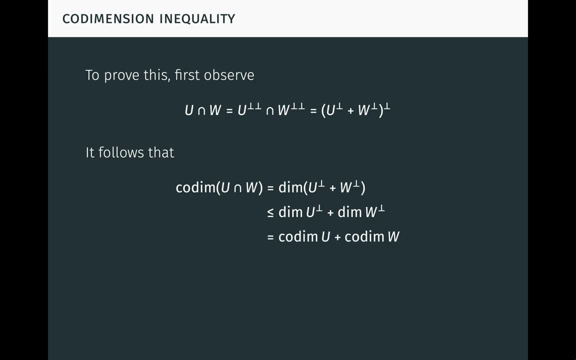 plus the dimension of w-complement, which is just the codimension of u plus the codimension of w. The dimension inequality can also be proved from the codimension inequality by similar reasoning. as you should verify, These inequalities exhibit duality. Each is obtained from the other by making certain syntactic substitutions. 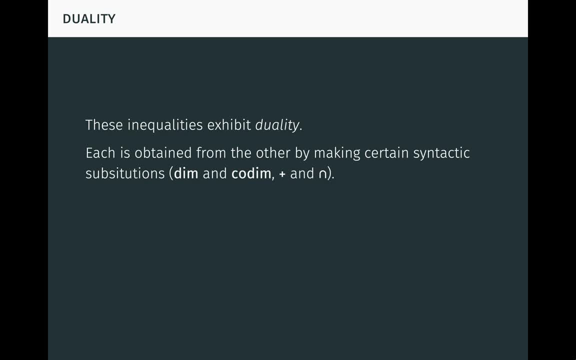 in this case swapping dimension and codimension and sum and intersection. Each is proved from the other by taking orthogonal complements under the inner product. In a certain sense, the inequalities are like mirror images of one another. We essentially get two inequalities for the price of one. And who doesn't like? 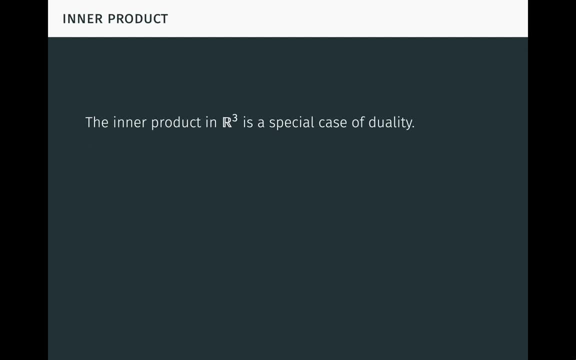 saving a few shekels on inequalities. But the inner product in R3 is just a special case of duality. Recall that it is bilinear, which means it is linear in each argument separately, as seen here. It is also nondegenerate, which means that if x times y is equal to zero for all y. 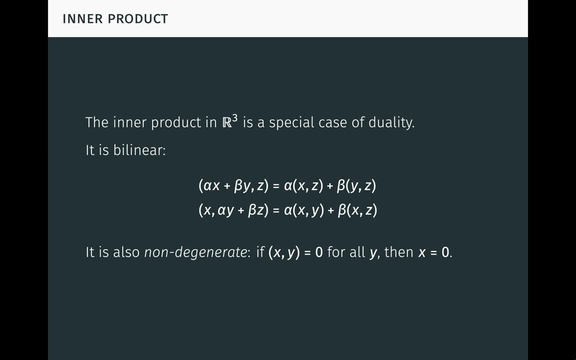 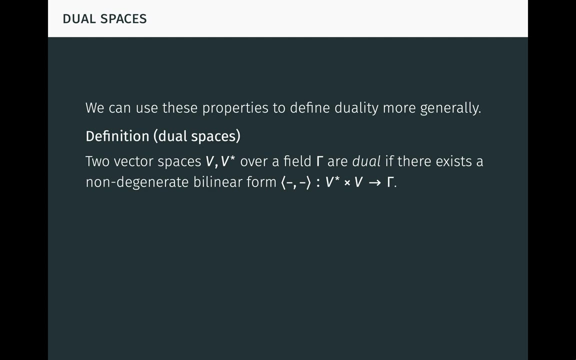 then x is equal to zero. And similarly, if y times x is equal to zero for all x, then y is equal to zero. We can use these two properties to define duality more generally. Two vector spaces, v and v-star, over a field gamma, are said to be dual if there exists a. 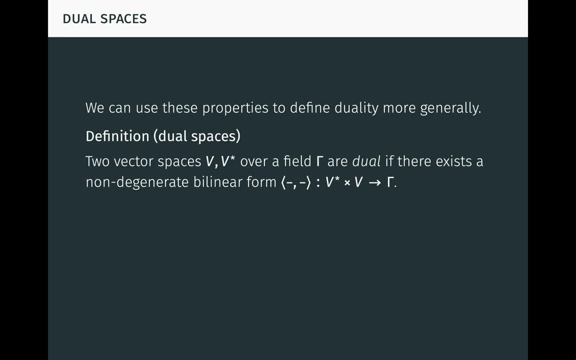 nondegenerate bilinear form, here denoted by angle brackets defined between them. The bilinear form is called the scalar product. The scalar product of a vector x-star in v-star and a vector x in v is denoted by x-star times x. 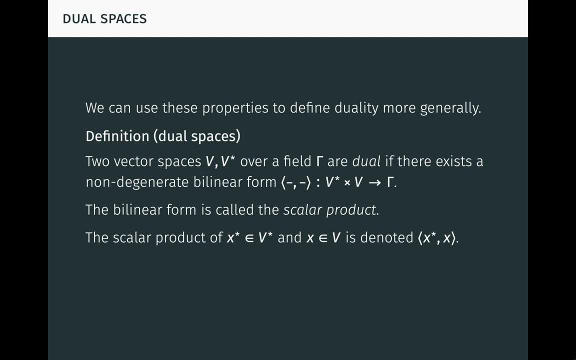 Here there is no relationship between x-star and x. x-star is an arbitrary vector in v-star and x is an arbitrary vector in v. Note that this definition is fundamentally symmetric between v and v-star, Although v-star appears on the left-hand side in the scalar product. we could just as soon use the 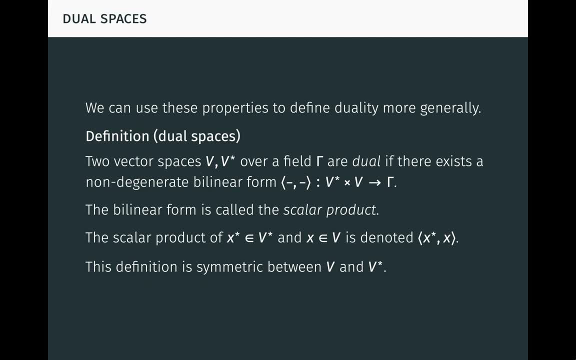 transposed scalar product where v-star appears on the right-hand side. We will exploit this symmetry extensively. If you've already seen duality somewhere else before, note in particular that v-star is not assumed to be the space of linear forms on v, I'll say more about that later. 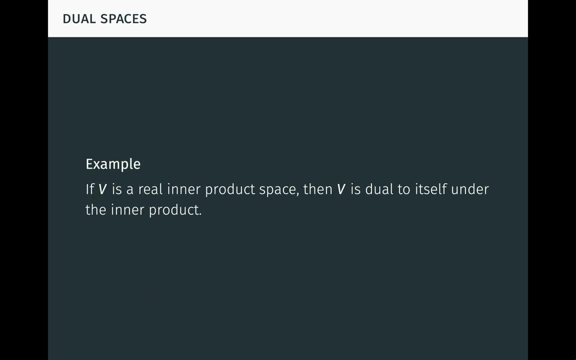 Let's now look at some examples of dual spaces. First, if v is a real inner product space, then v is dual to itself under the inner product, as we've already seen in the case of R3.. The question naturally arises: what about complex inner product spaces? 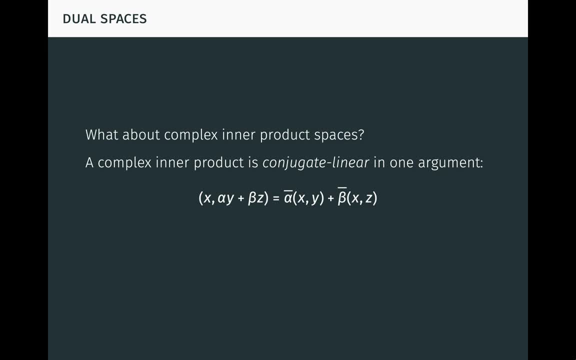 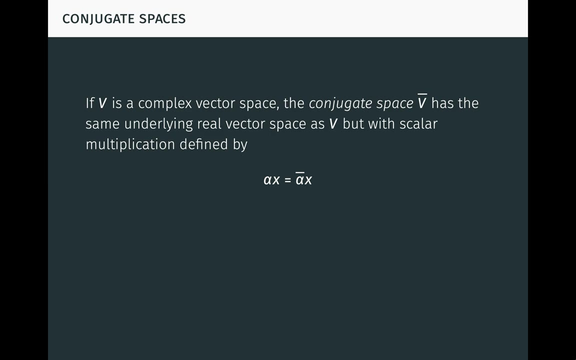 Recall that a complex inner product is conjugate linear in one argument, as seen here. So technically it is not a scalar product. However, we can work around this issue. If v is a complex vector space, the conjugate space, v conjugate, has the same underlying real vector space as v. 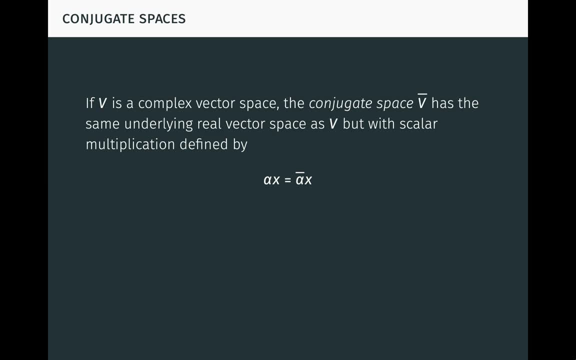 but with scalar multiplication defined using complex conjugation. Here the left-hand side is scalar multiplication in v conjugate, while the right-hand side is scalar multiplication in v. The identity map: kappa from v to v conjugate is then conjugate linear, because kappa of alpha x plus beta y is alpha conjugate. kappa x plus beta conjugate. kappa y. 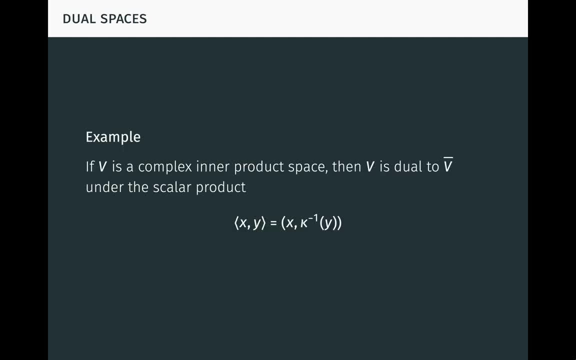 as you should verify. Now, if v is a complex inner product space, then v is dual to v conjugate under the scalar product defined here. Notice how the conjugate linearity of kappa counteracts the conjugate linearity of the inner product to produce a scalar product. In this case, two wrongs really do make a right. 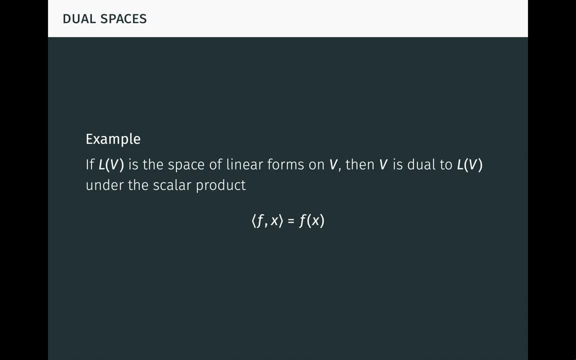 As another important example, if Lv is the space of linear forms on v, that is, the space of linear maps from v into the base field, gamma, then v is dual to Lv under the scalar product, where f times x is just f of x. It's worth pausing the video to think through why. 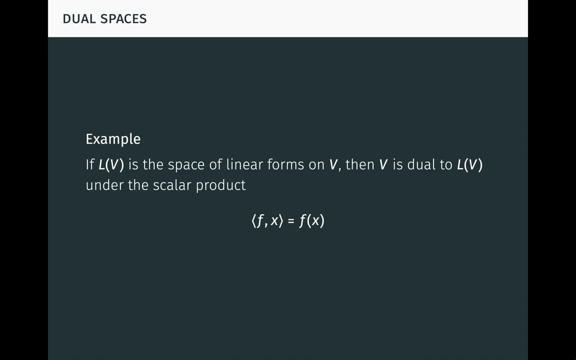 this really is a scalar product. If you're interested in learning more about the linear forms that you can find, then think about the expression f, as f is a non-degenerate bilinear form. In a certain sense, linear forms are a universal example. 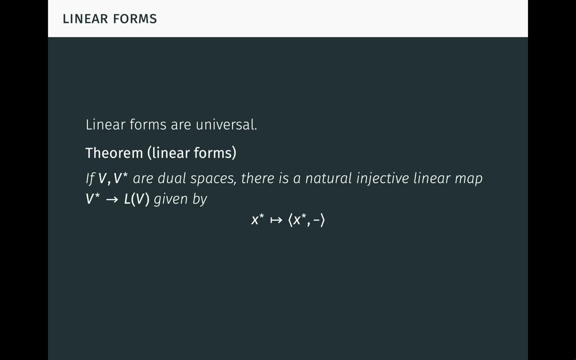 If v and v star are dual spaces, there is a natural injective linear map from v star to Lv, given by sending a vector x star to the linear form x star times blank. This linear form takes in a vector x in v and returns the scalar product x star times x. If v is finite dimensional. 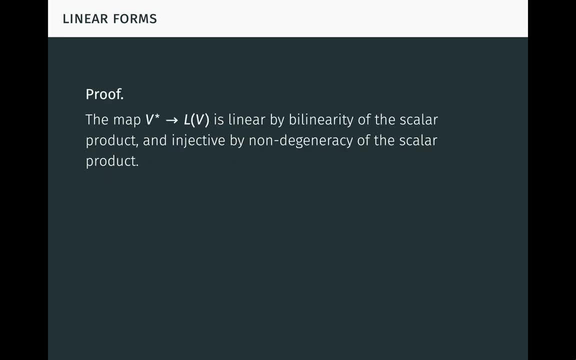 the map is an isomorphism. If v is finite dimensional, the map is an isomorphism. To see why this is true, first observe that the map from V-star to L-V is linear by bilinearity of the scalar product and injective by nondegeneracy of the scalar product. 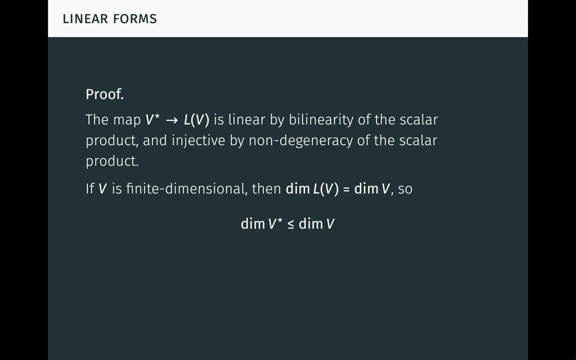 If V is finite-dimensional, then we know that the dimension of L-V is equal to the dimension of V. so by injectivity of the map, the dimension of V-star is at most the dimension of V. In particular, V-star is also finite-dimensional. 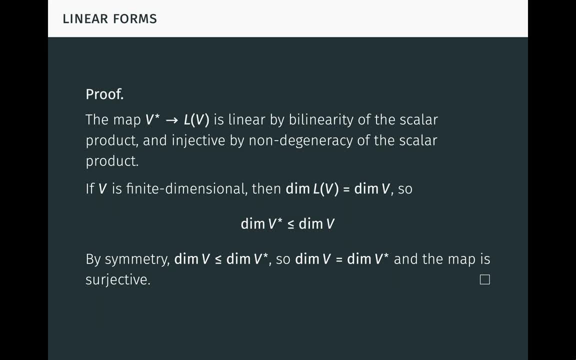 By symmetry of duality, it follows that the dimension of V is at most the dimension of V-star. so the dimension of V is equal to the dimension of V-star and the map is surjective. Of course there is also a map from V to L-V-star, given by sending a vector x to the linear. 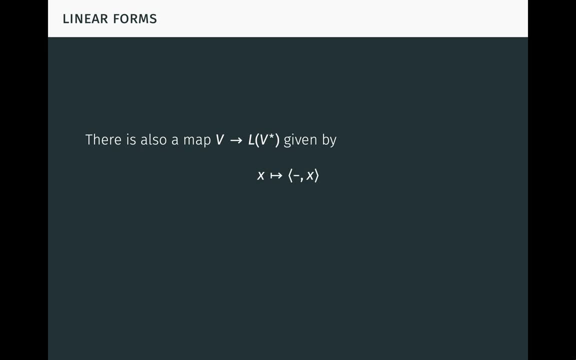 form blank times x. But it's important to see that this theorem does not give us a natural map from V to L-V. In general, V is not naturally isomorphic to L-V, even when V is finite-dimensional. So what is the natural map? 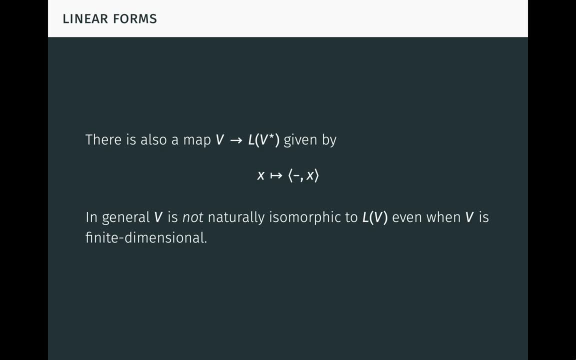 We will see a special case where this is true in just a moment. however, It follows from the theorem that if V is finite-dimensional and V-star and V-star are both dual to V, there is a natural isomorphism from V-star to V-star which preserves the scalar product. 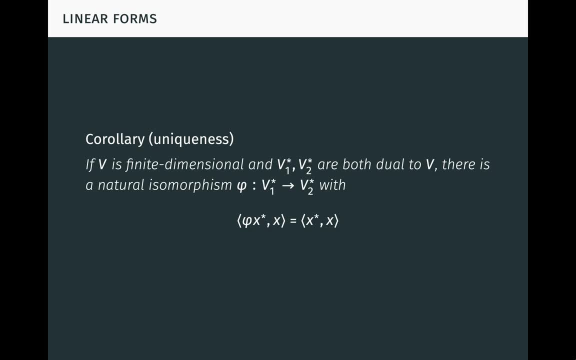 This means that a finite-dimensional dual space is unique up to unique isomorphism. In particular, if V is finite-dimensional, then since V is dual to L-V and V-star is finite-dimensional, then since V is dual to L-V, it follows that there is a natural 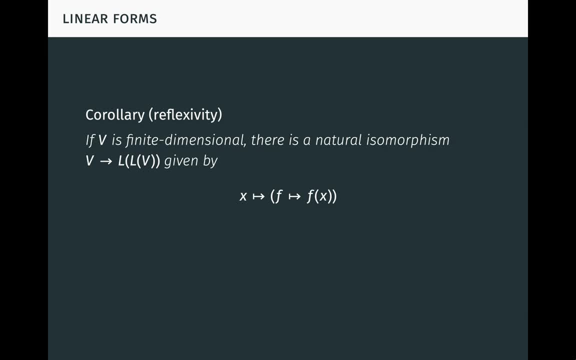 isomorphism from V to L-L-V, given by sending a vector x to the linear form which evaluates linear forms at x. This is called reflexivity and means that a vector x can be naturally identified with the linear form evaluation at x. Now why would we ever want to do this? 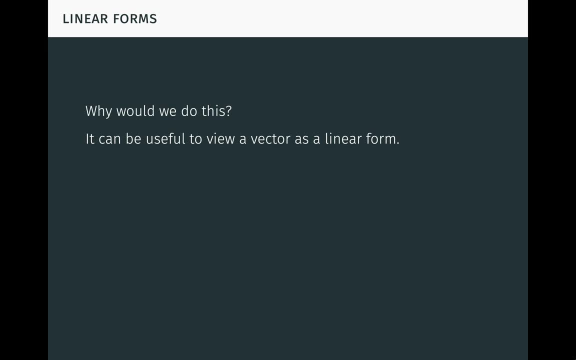 Well, it can be useful to view a vector as a linear form. In fact, in many treatments of duality which do not apply to linear form, we can simply identify a vector as a linear form. However, if we do this, we can also evaluate the vector as a linear form. 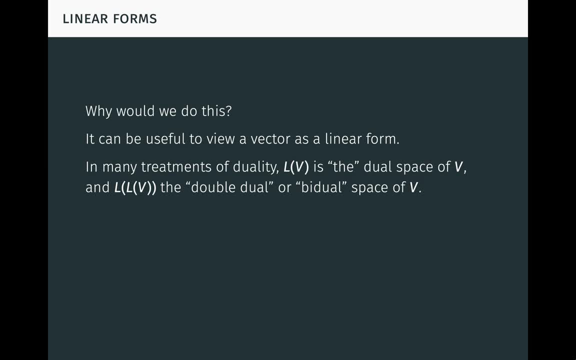 not use our definition of dual space. LV is the singular dual space of V and LLV is the double, dual or bi-dual space of V. If V is finite-dimensional, then V is identified with LLV by reflexivity. to establish symmetry of the duality relation between V and LV By 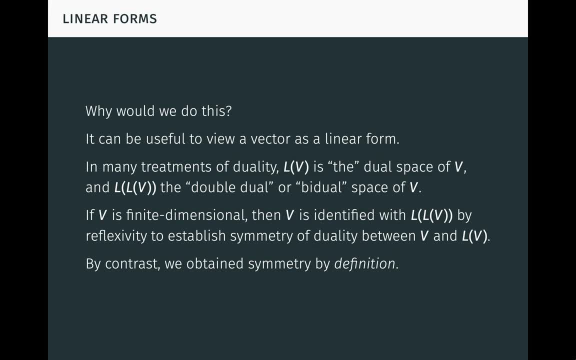 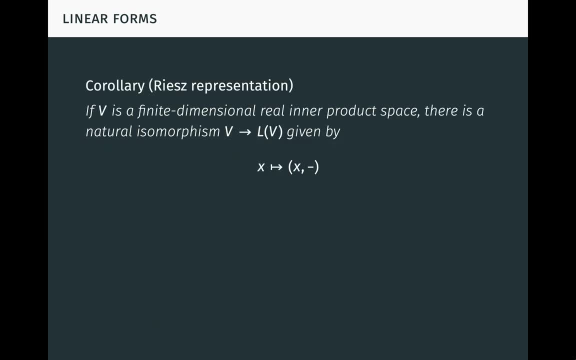 contrast, we obtain symmetry by definition. Ours is certainly the better approach here, and anyone who thinks otherwise is a crazy person. In the case of a finite-dimensional real inner product space, we do obtain from the theorem a natural isomorphism from V to LV, given by sending a vector x to the linear form x times. 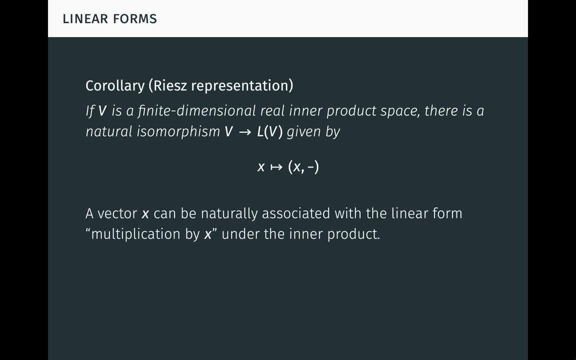 blank under the inner product. This means a vector x can be naturally associated with the linear form multiplication by x. This linear form is called the covector of x and is very useful in many applications. A similar result holds in the complex case. 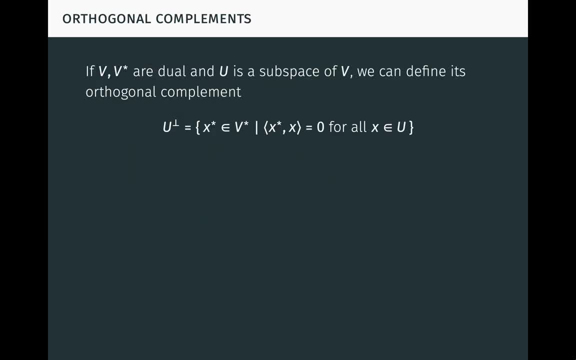 Moving on, If V and V-starr are dual spaces and U is a subspace of V, we can define its orthogonal complement in the obvious way. Note U complement is a subspace of V-starr. By symmetry we can also take complements of subspaces of V-starr to obtain subspaces of V. 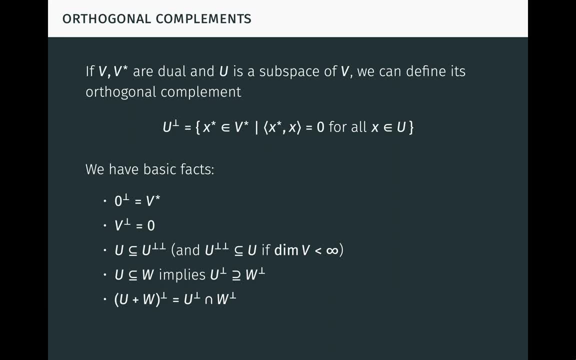 We have a number of basic facts similar to the ones we saw earlier in the special case of Ar, although not everything carries over to the infinite-dimensional case. For every fact here is a corresponding fact for subspaces of V and V-starr in the obvious. 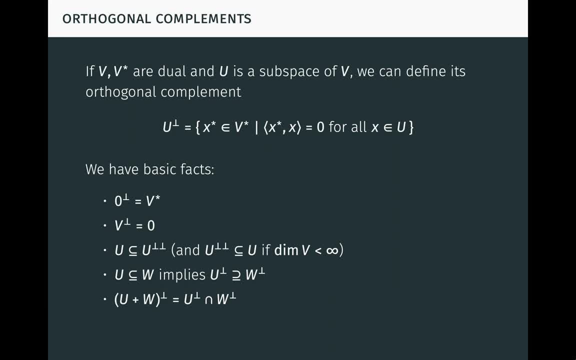 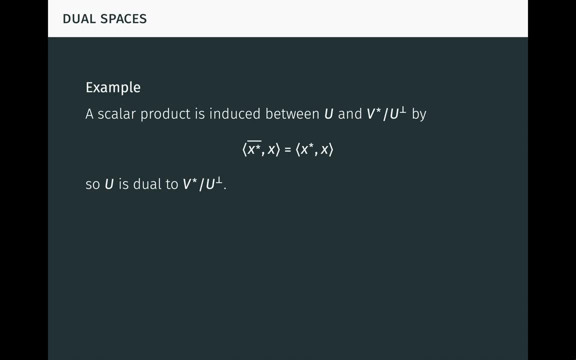 way, If V is редistinguished, then U is a subsequence of V-starr, in the obvious way for subspaces of V-star, again by symmetry. This leads to another important example. A scalar product is induced between the subspace U and the quotient space V-star. mod U complement 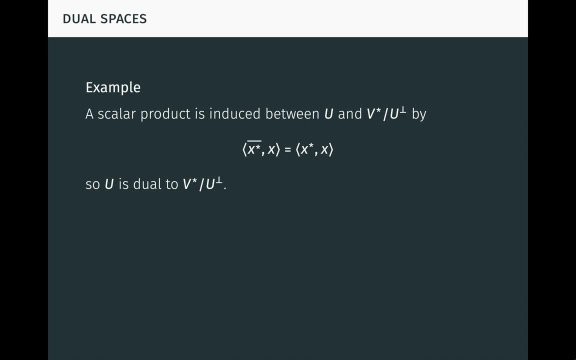 by the rule seen here, where the bar denotes projection. So U is dual to V-star mod U complement. It's worth pausing the video to verify that this really is a well-defined non-degenerate bilinear form. This means that subspaces are dual to quotient spaces. 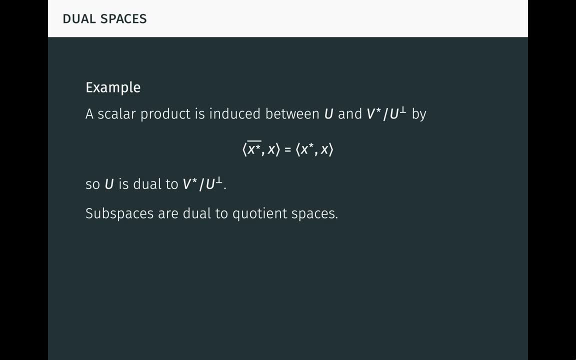 Every fact about subspaces can be translated into a corresponding fact about quotient spaces, and vice versa. This is extremely useful, because it may be easier to see that a certain fact is true of quotient spaces, say, and then translate that to a fact about subspaces rather than prove. 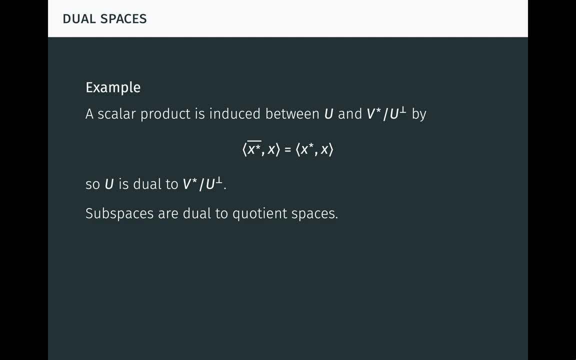 the fact about subspaces directly. We saw something similar with the codimension inequality for intersections in R3 earlier. If V is finite-dimensional, it follows from this example that the dimension of U plus the dimension of U complement is equal to the dimension of V, which remains a fundamental fact. 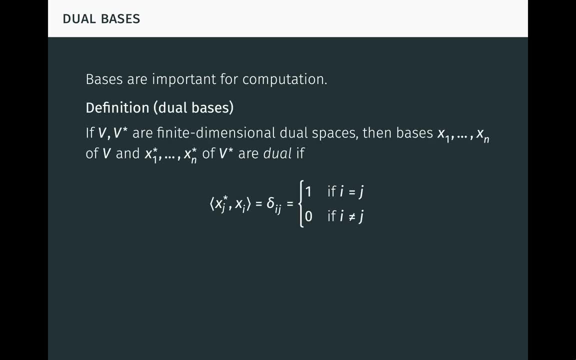 Bases are extremely important for computation. If V and V-star are finite-dimensional dual spaces, then bases x1 to xn of V and x-star 1 to x-star n of V-star are dual. if x-star j times xi is equal to delta ij, which is 1 when i equals j, 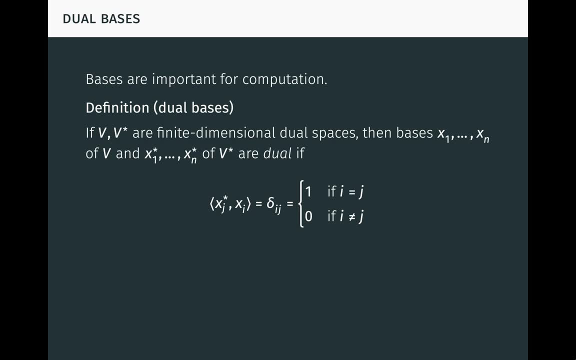 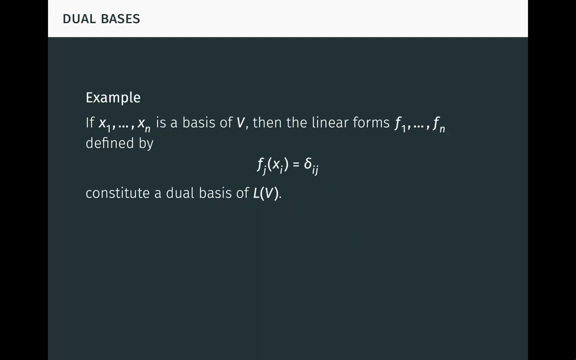 and 0. otherwise That delta is called the Kronecker delta. Note: this definition is symmetric between the two bases. It's immediate from nondegeneracy of the scalar product that the dual basis is unique if it exists. As an example, if x1 to xn is a basis of V, 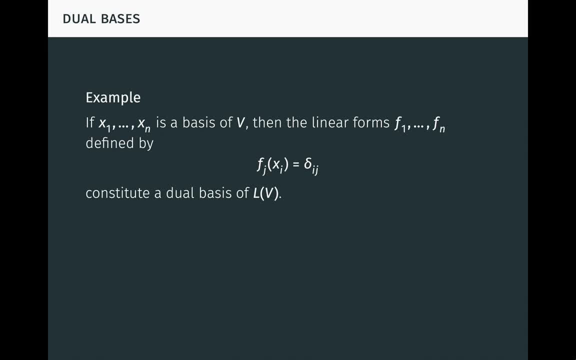 then the linear forms f1 to fn, defined by fj of xi equals delta ij, constitute a dual basis of LV. as you should verify, It follows from this example and the theorem on linear forms that a dual basis always exists And by symmetry every basis is a dual basis. But remember, we're only talking about the finite-dimensional case. 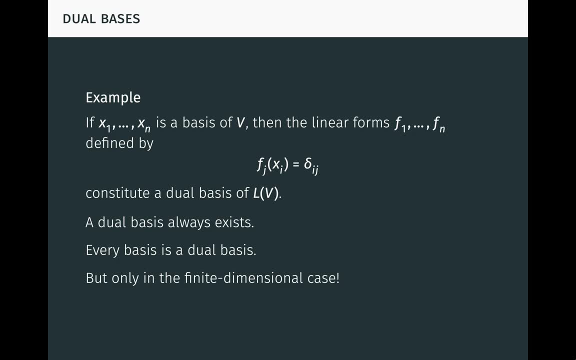 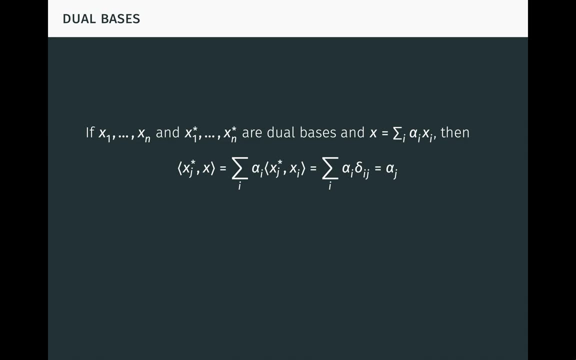 here. These facts don't carry over to the infinite-dimensional case. If x1 to xn and x-star 1 to x-star n are dual bases and x is the sum over i of alpha i, xi, then x-star j times x is just alpha j. This means a vector's components with 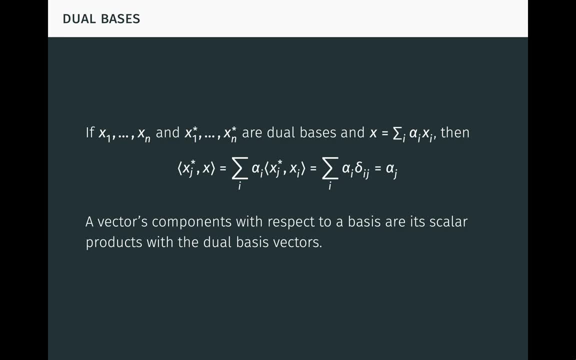 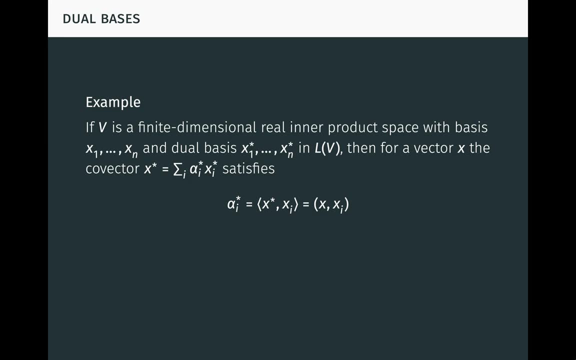 respect to a basis are just its scalar products, with the dual basis vectors As an example. if V is a finite-dimensional real inner product space with basis x1 to xn and dual basis x-star 1 to x-star n in LV, then for a vector x, the covector x-star. 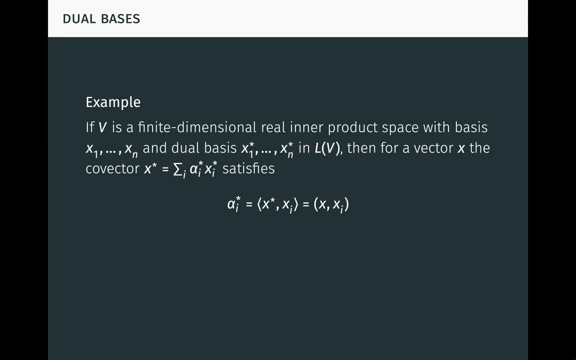 equal to the sum over i of alpha-star i. x-star i satisfies alpha-star i equals the scalar product of x-star and xi, which is just the inner product of x and xi. In other words, a covector's components with respect to a dual basis are just the. 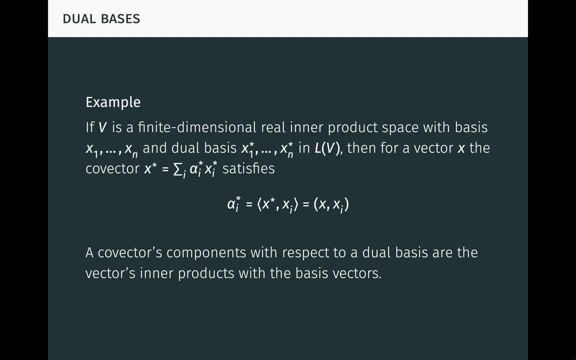 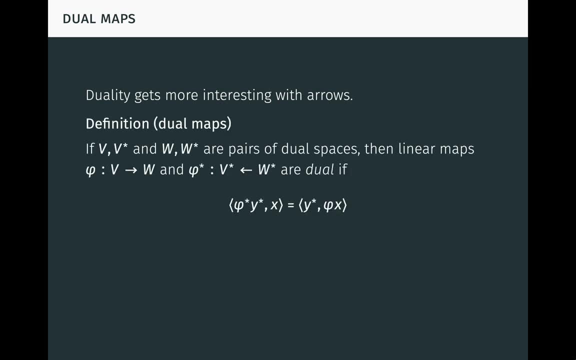 vector's inner products. with the basis vectors. Duality gets more interesting with arrows, that is, linear maps. If v- v-star and w- w-star are pairs of dual spaces, then linear maps- phi from v to w and phi-star to v-star from w-star- are 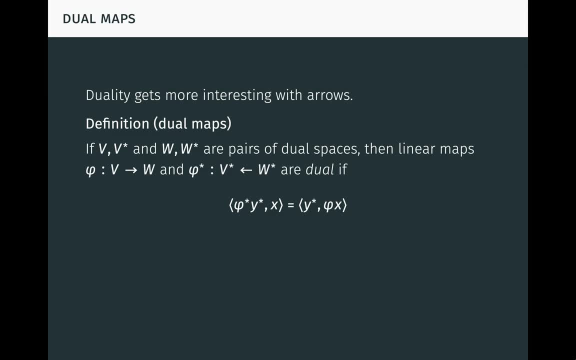 dual if they satisfy this relation instant only, as lar Oksi Demunizilgians were fairly numerous on the internet during their final state. Phi-star y-star times x equals y-star times x equals y-star over y-prozятich sentence items: Question 2.. 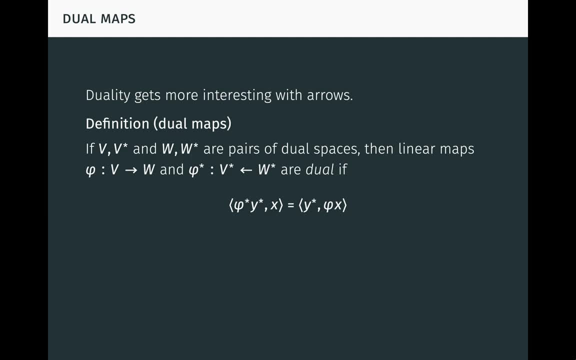 y star times, phi x for all, y star in w star and x in v. I'll say more about this relation in a second, but first notice the arrow is reversed between phi and phi star, like a mirror image, Also like the definition of dual space. this definition is fundamentally 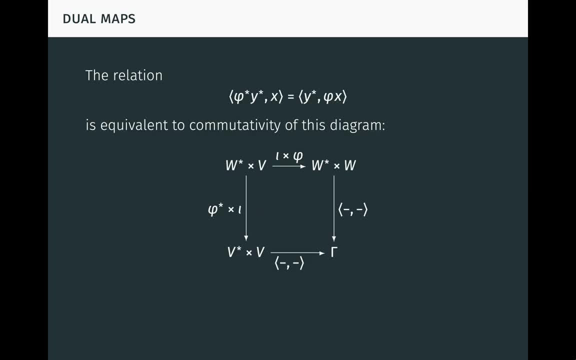 symmetric between phi and phi star. The relation in the definition is equivalent to commutativity of this diagram, which helps to visualize the situation and also to see how one might arrive at the relation by thinking about the possible interactions of linear maps and scalar products. It's immediate from nondegeneracy of the scalar product that a dual map is unique. 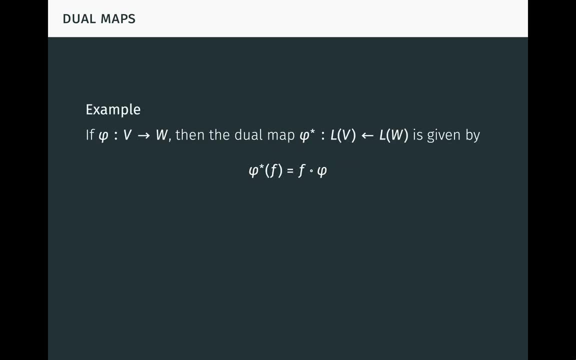 if it exists. As an example, if phi is a linear map from v to w, then the dual map phi star to lv, from lw is given by pre-composition of phi. This can be visualized in this diagram. It follows from this example and the theorem on linear forms that a dual map always 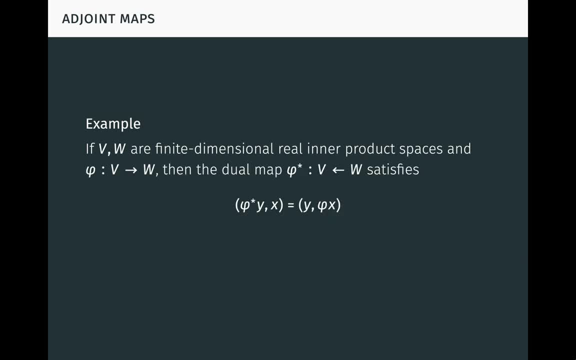 exists in the finite-dimensional case. As another example, if v and w are finite-dimensional real inner product spaces and phi is a linear map from v to w, then the dual map phi star to v from w satisfies phi star. y times x equals y times phi x under the inner products for all, y in w and x in v. Therefore phi star. 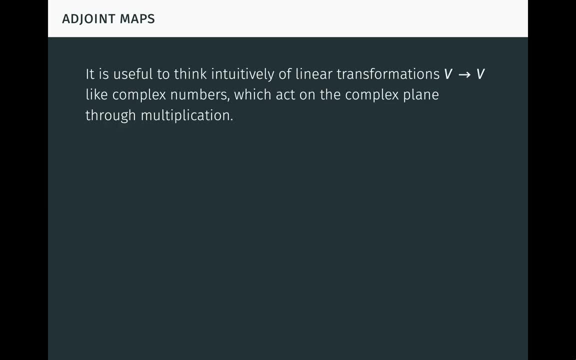 is just the familiar adjoint of phi. In this context, it's useful to think intuitively about the relation between phi, star and lv. In this context, it's useful to think intuitively about the relation between phi, star and lv. Firstly, we can see that the linear transformations on v are similar to complex numbers which 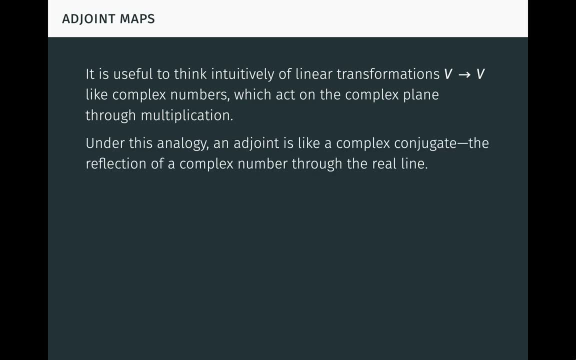 act on the complex plane through multiplication. Under this analogy, an adjoint is like a complex conjugate—the reflection of a complex number through the real line. This analogy is strong and leads to important parallels between classes of linear transformations and classes of complex. 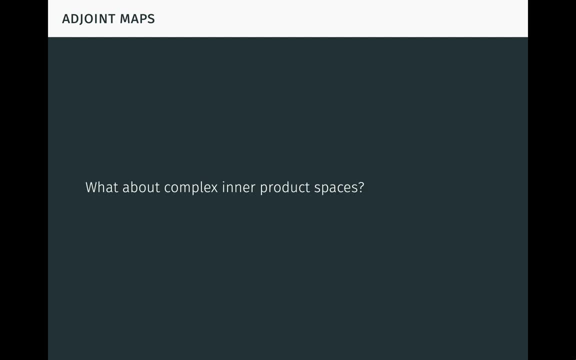 numbers as seen in this beautiful table. What about complex inner product spaces? If v and w are finite-dimensional complex inner product spaces, then phi, star and lv are the same. In this example, phi, star and and. phi is a linear map from V to W. then there is a dual map: phi star to V, conjugate from W. 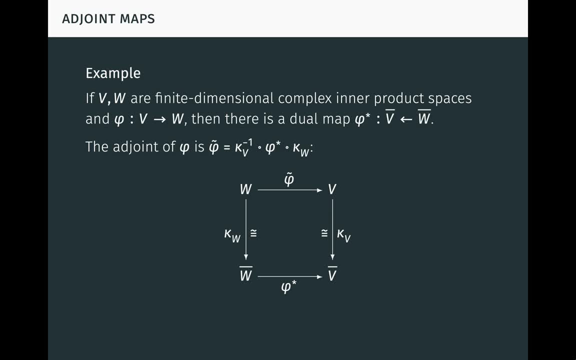 conjugate. The adjoint is just the conjugate of the dual by the conjugate linear identity maps as seen in this commutative diagram. So in the complex case the adjoint is almost the dual, like the inner product is almost the scalar product. 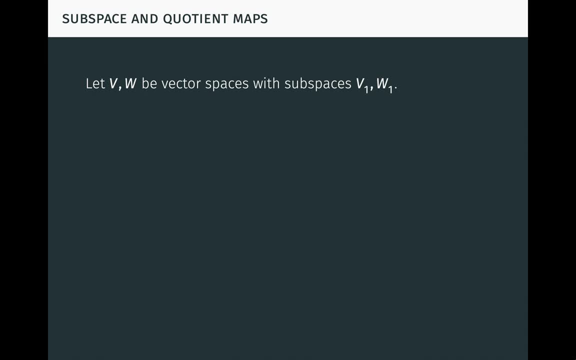 Now let V and W be vector spaces with subspaces V1 and W1.. If phi is a linear map from V to W which maps V1 into W1, there are induced subspace and quotient maps, phi1 from V1 to W1,. 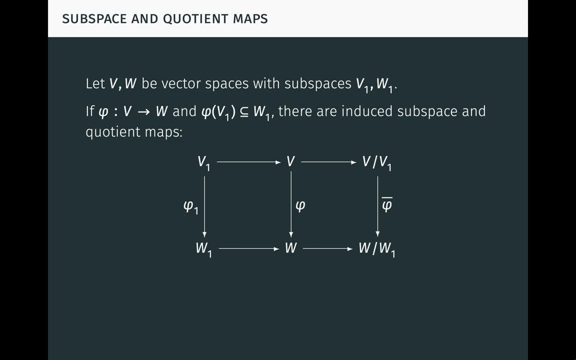 and phi bar from V mod V1 to W mod W1, making this diagram commute Here: phi1x equals phix for all x in V1, and phi bar x bar equals phi x bar for all x in V, where the bars denote projection. 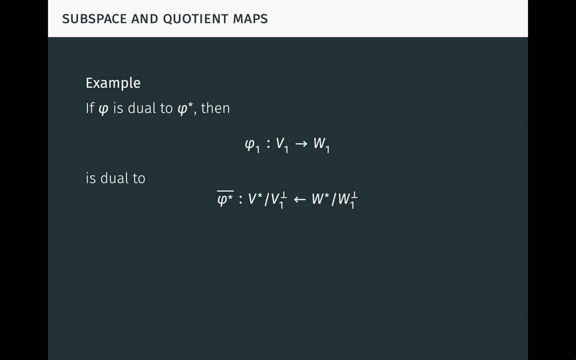 This leads to another important example. If phi is dual to phi star, then phi1 from V1 to W1 is dual to phi star. bar to V star mod V1 complement from W star mod W1 complement. This extends our previous example which showed that subspaces are dual to quotient. 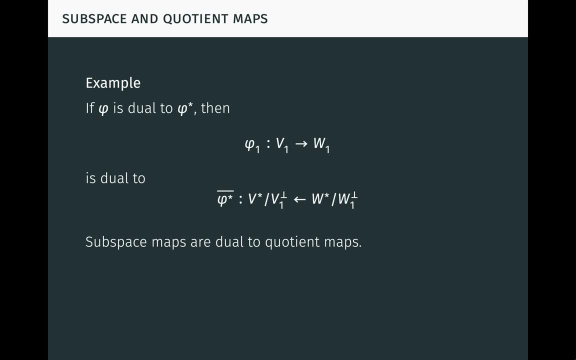 spaces by showing that subspace maps are dual to quotient maps. In particular, the canonical injection from V1 into V is dual to the canonical projection onto V star mod V1 complement from V star. The star operation has several basic properties. If phi phi star and psi psi star are dual maps. 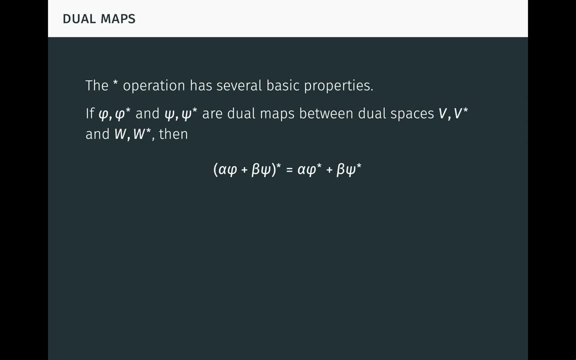 between dual spaces V? V star and W? W star, then alpha phi plus beta psi has the dual alpha phi star plus beta psi star. If omega, omega star are also dual maps between the dual spaces W? W star and x? x star, then omega after phi has the dual phi star after omega star. Note the order reversal here. 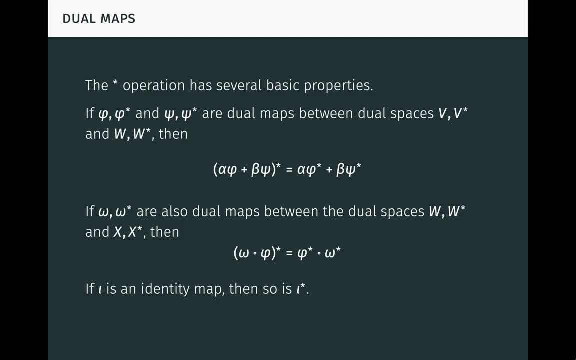 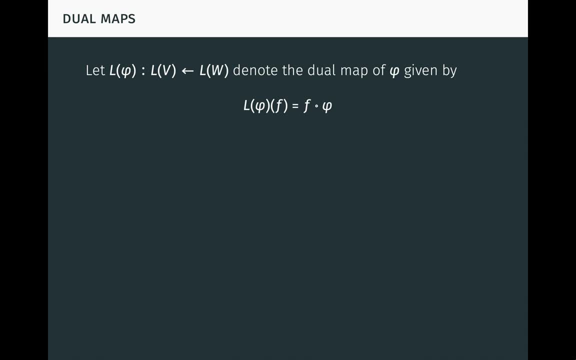 Finally, if iota is an identity map, then so is iota star. Now let L phi to L V from L W denote the dual map of phi given by precomposition. Then these results show that L is linear and L reverses composites. 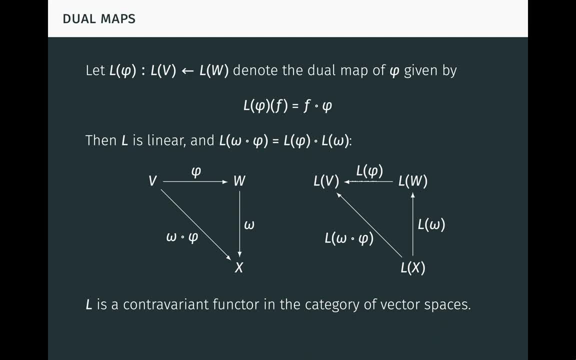 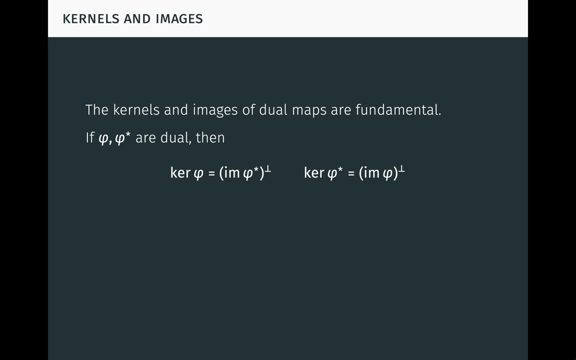 Since L also preserves identity maps, it follows that L is a contravariant functor in the category of vector spaces. To learn more about functors, see my other videos about category theory. The kernels and images of dual maps are fundamental. If phi and phi star are dual, then it's 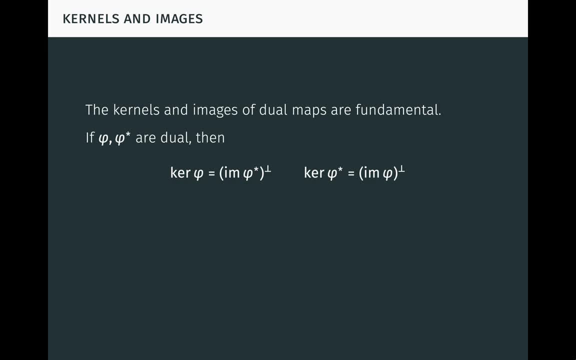 easy to see that the kernel of phi is the complement of the image of phi star and, by symmetry, the kernel of phi star is the complement of the image of phi. In the finite dimensional case, we can take complements of both sides of these equations to obtain: 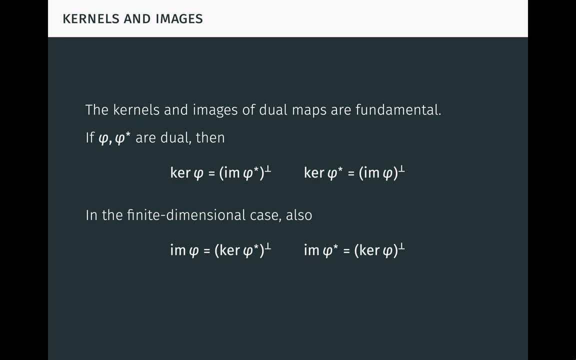 that the image of phi is the complement of the kernel of phi star and the image of phi star is the complement of the kernel of phi. socks have many important applications, but we will look at just a few First. if phi maps from: 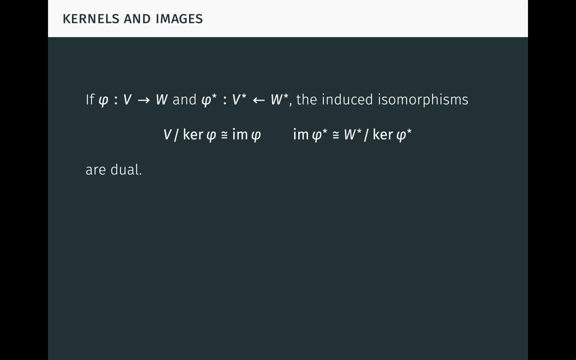 v to w and the dual map phi star maps to v star from w star. then the induced isomorphisms from v mod, the kernel of phi, to the image of phi and to the image of phi star, from w star mod, the kernel of phi star, are dual. Second, if v is finite dimensional, it follows: 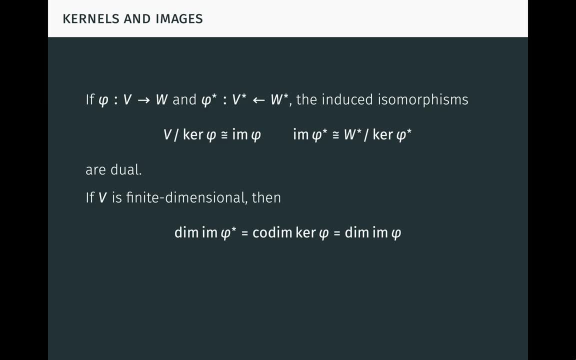 that the dimension of the image of phi star is just the codimension of the kernel of phi, which is just the dimension of the image of phi by the rank-nullity theorem. Therefore, the rank of phi star equals the rank of phi. Let v and v star be finite dimensional dual spaces, If phi and phi star are dual transformations. 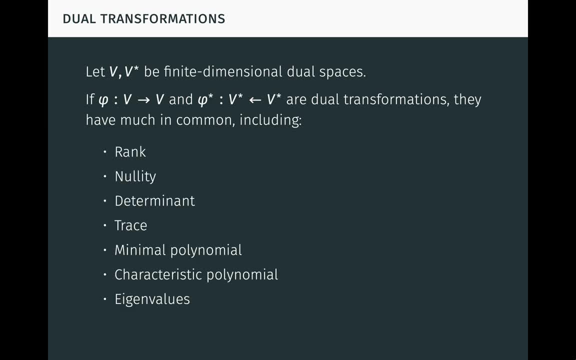 on v and v star. they have much in common, including rank, as we just saw: nullity, determinant trace, minimal polynomial, characteristic, polynomial eigenvalues and more. It becomes clear that the rank of phi star is just the codimension of the image of phi. by the rank, 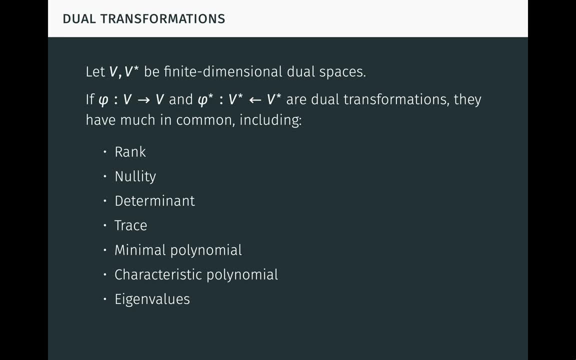 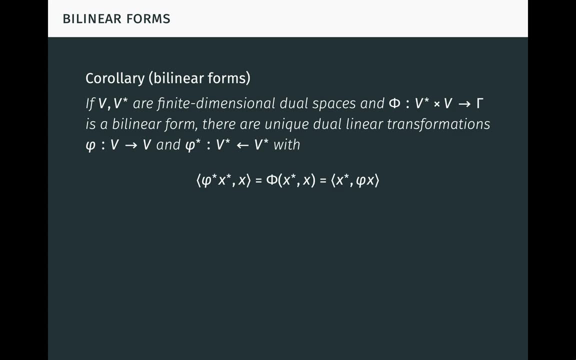 of v star. They also share a common bilinear form. We obtain as another corollary of the theorem on linear forms that if v and v star are finite dimensional dual spaces and phi is a bilinear form between them, then there are: 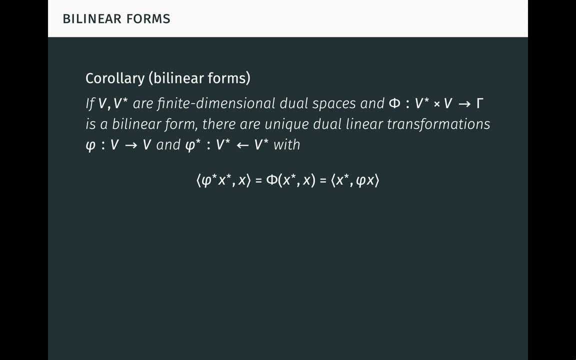 unique dual linear transformations phi on v and phi star on v star, which represent the bilinear form through the scalar product. This correspondence induces natural isomorphisms between the space of bilinear forms and the spaces of linear transformations on v? star and v. 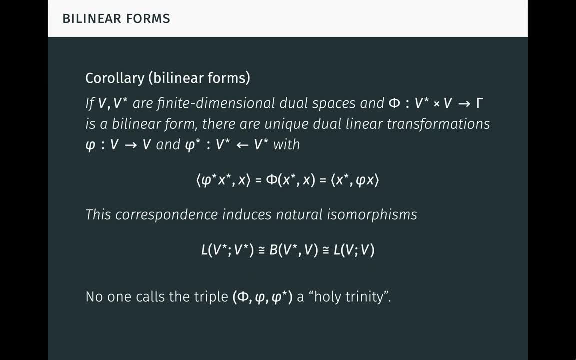 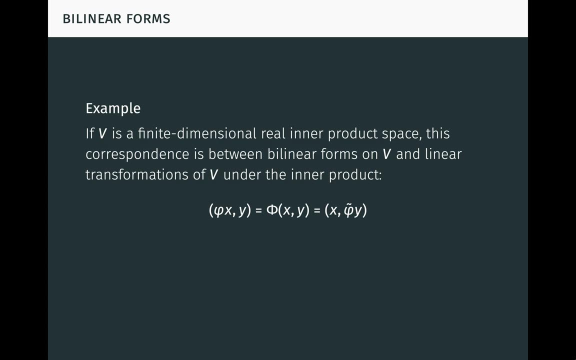 It's worth noting that, despite the strong resemblance, no one calls the triple phi phi phi star a holy trinity. Nevertheless, after watching this video, I hope you have the witness of the dual transformation in your heart. If v is a finite dimensional, real inner product space, this correspondence is between bilinear. 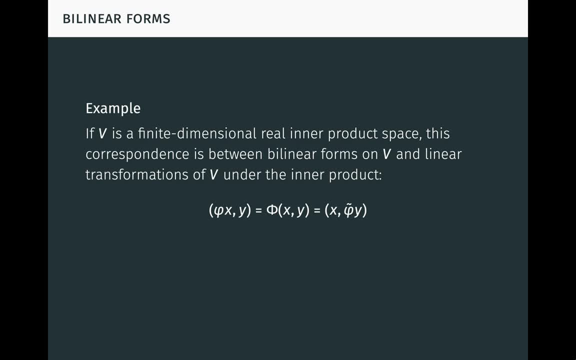 forms on v and linear transformations of v under the inner product Properties of the bilinear form correspond to those of the transformations like symmetry, skew symmetry and so on, with some mild assumptions on the ground field. This is one reason why the study of bilinear forms and associated quadratic forms is so central in linear algebra. 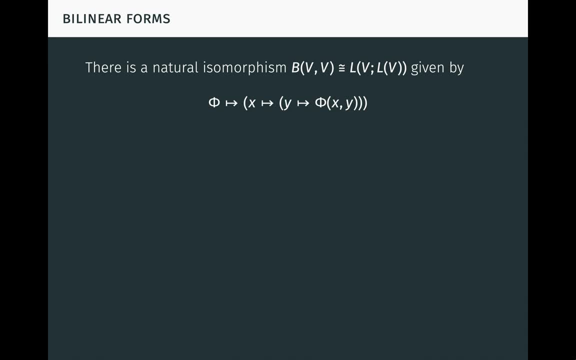 In this context, there is also a natural isomorphism from the space of bilinear forms on v to the space of linear transformations, from v into the space of linear forms on v, given by currying the bilinear forms. This allows us to write phi of x- y as phi of x of y. 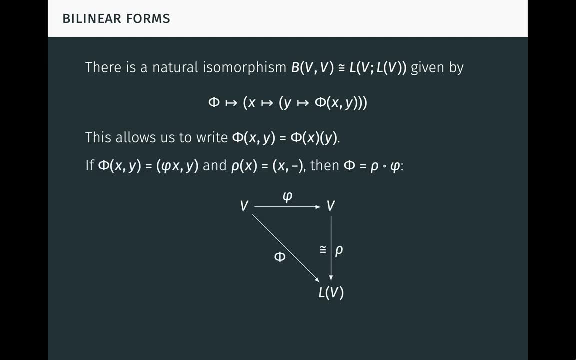 Now, if the bilinear form phi corresponds to the linear transformation phi, then the pair is connected by the Riesz representation as seen here. If we instead curry y first instead of x, then we obtain a similar connection involving phi adjoint instead of phi. 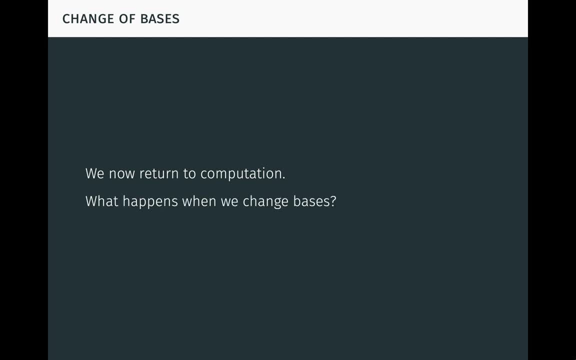 We return now to computation. Specifically, what happens when we change bilinear forms? We return now to computation. Specifically, what happens when we change bilinear forms and associated quadratic forms? We return now to computation. Specifically, what happens when we change the basis? 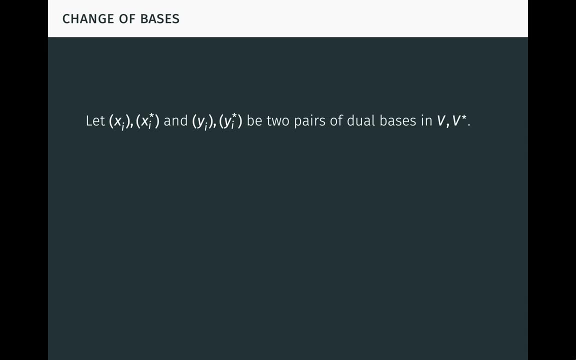 Let xi- x-star-i and yi- y-star-i be two pairs of dual bases in Vv-star. If tau is a linear transformation of v, then we know tau-star y-star j times xi equals y-star j times tau xi. It follows immediately that tau maps from the x's to the y's. if 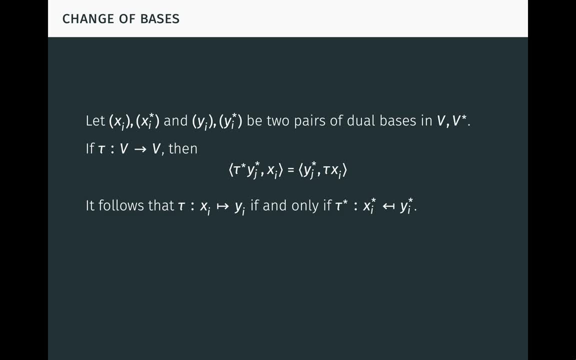 and only if tau-star maps to the x-stars from the y-stars. We return now to computation. basis in a space is contragradient to change of dual basis in a dual space. As an example, let V be a finite-dimensional real inner product space. If basis vectors 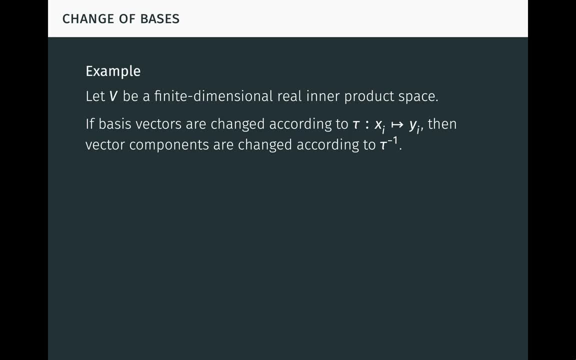 are changed according to tau, then we know that vector components are changed according to tau. inverse, Due to contragradients, covector components are changed according to tau, as we can see here. For this reason, the covector components are called covariant components. 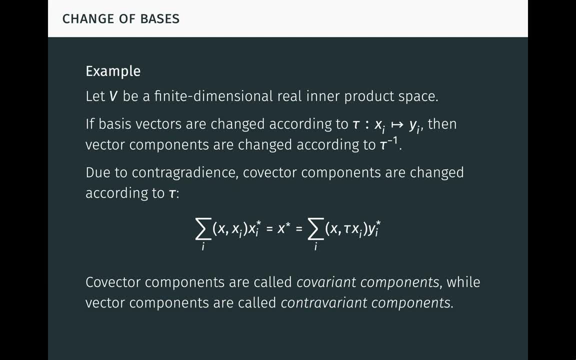 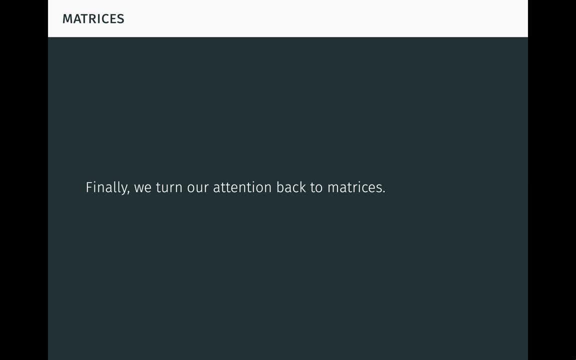 while the vector components are called contravariant components. This covariance is one of the properties that makes covectors useful in applications. Finally, we turn our attention back to matrices. Let xi- x-star, i be dual bases in V- v-star, and let yi- y-star, i be dual bases in W- w-star. Then we have a theorem, If phi, from V to W. 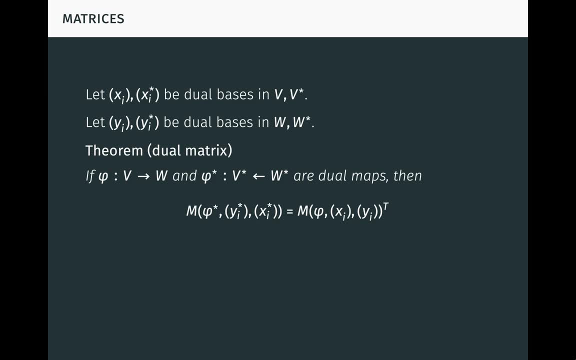 and phi-star to V-star, from W-star, are dual maps, then the matrix of phi-star with respect to the y-stars and the x-stars is the transpose of the matrix of phi with respect to the x's and the y's. More succinctly, the matrix of a map with 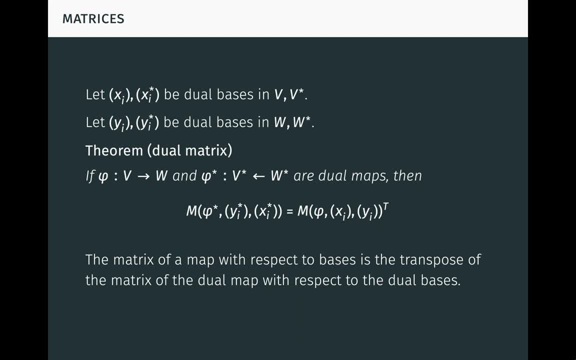 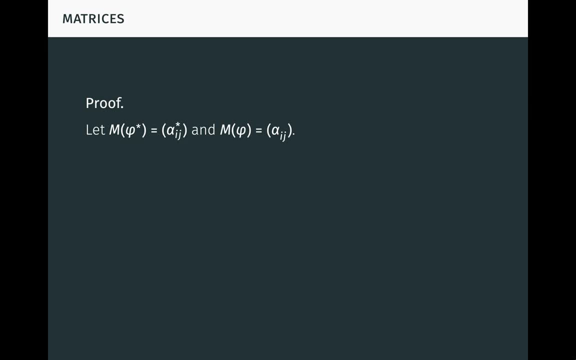 respect to bases is the transpose of the matrix of the dual map with respect to the dual bases. The proof is straightforward. Let the matrix of phi-star be alpha-star ij and the matrix of phi be alpha-ij, where for both the alpha-stars and the alphas, the first index counts rows. 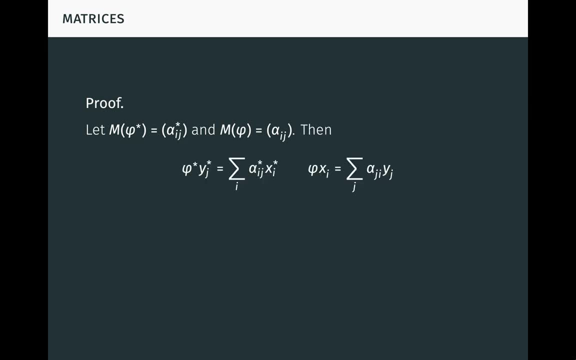 and the second index counts rows. Then by definition we have these expressions for phi-star and phi. It follows that alpha-star ij is equal to alpha-ji, so the matrices are transposed. It's worth noting that sometimes in linear algebra, for example when working with tensors, 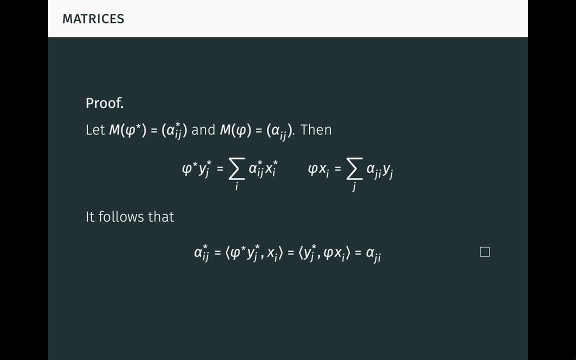 or with modules over possibly non-commutative rings. it's common to adopt a transpose convention for matrices in dual spaces. If this is done, the theorem then states that dual maps have the same matrix. However, in either case, transposition is happening. 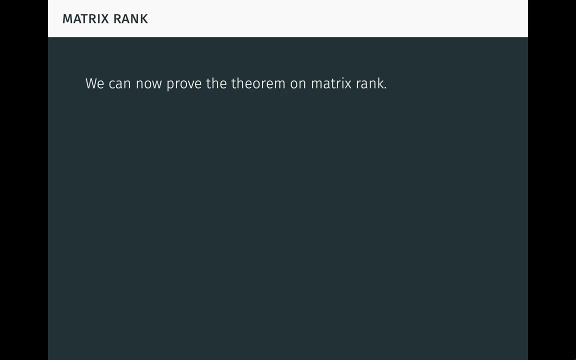 somewhere. With this result in hand, we can now prove the theorem on matrix rank from earlier. If m is a matrix, then m induces a linear map through left multiplication of column vectors. It's easy to see that the column rank of m is the rank of this map.